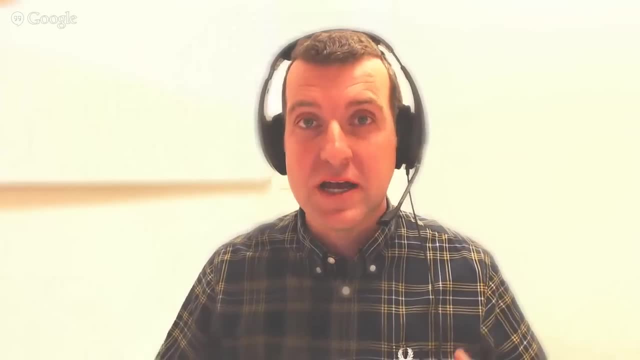 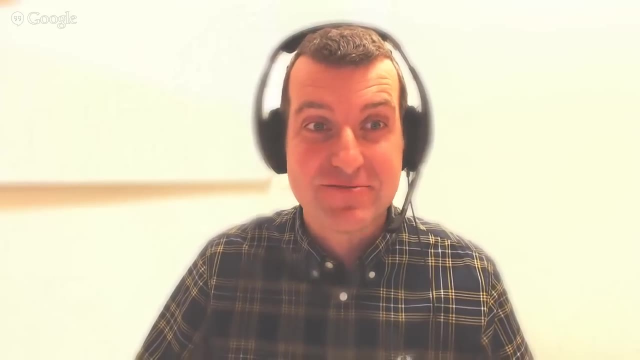 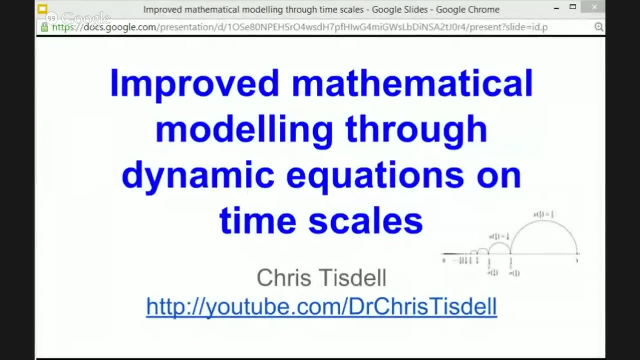 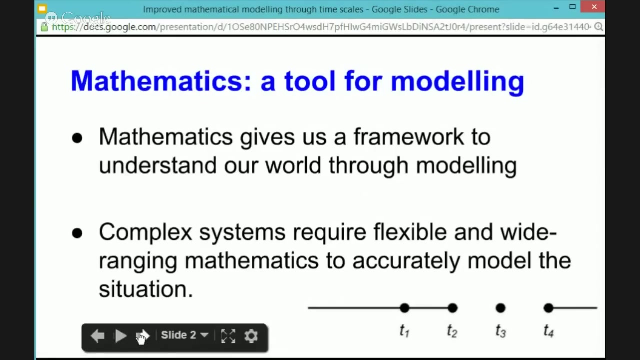 Dynamic equations on timescales. This is a very low-level talk. You don't need any mathematics to understand this talk and it'll be a short one, So let me share my screen with you and I can share some ideas. Improved mathematical modelling through dynamic equations on timescales. So what does that mean? Well, we all know that mathematics is something beautiful. It can be studied in its own right. 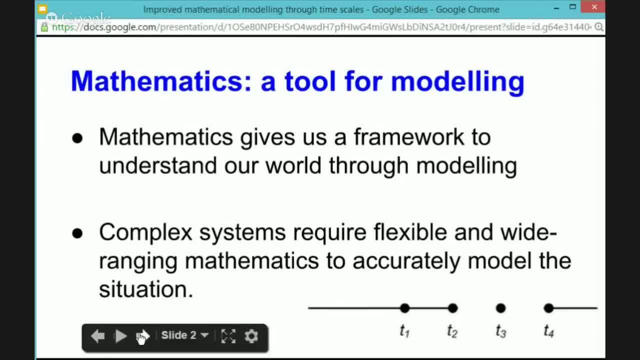 But it's also an important tool for modelling And, in particular, it gives us a framework to understand the world around us and the dynamical things in our world. These sorts of very complicated phenomena require a framework that's flexible and wide-ranging in the mathematical sense. 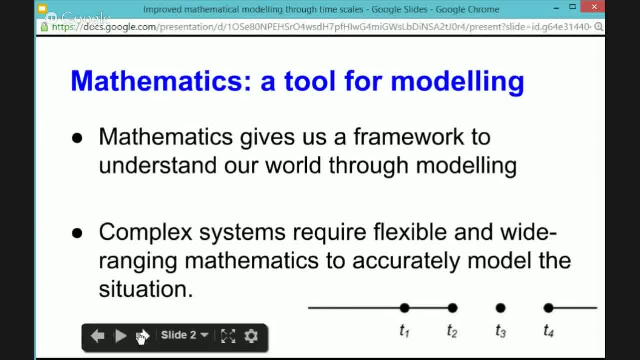 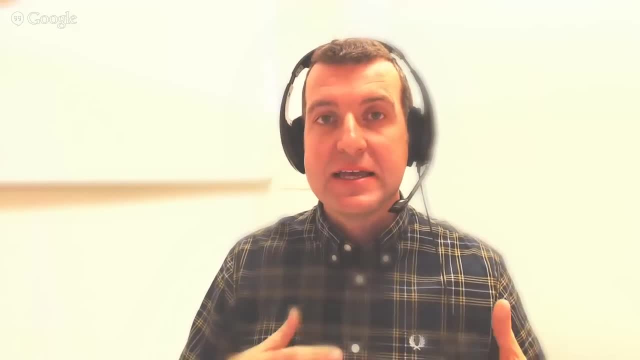 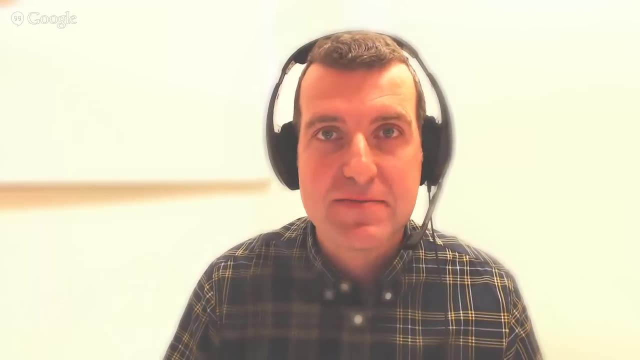 The greater the flexibility and the more wide-ranging the mathematics, the more accuracy we will get To model the situation. Now this area- dynamic equations on timescales- is very, very flexible And it sort of extends and combines different parts of mathematics to really give a wide-ranging modelling experience. 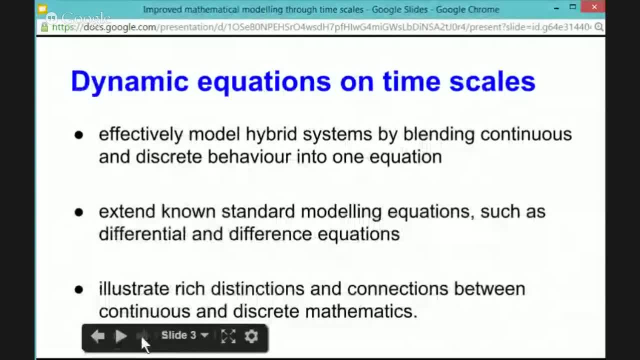 So what do I mean by that? Let me show you Now dynamic equations on timescales. they effectively model hybrid systems- And when I say hybrid systems, I'm talking about systems or phenomena that have continuous elements and discrete elements. And these dynamic equations on timescales? they harmoniously blend the continuous and the discrete together. 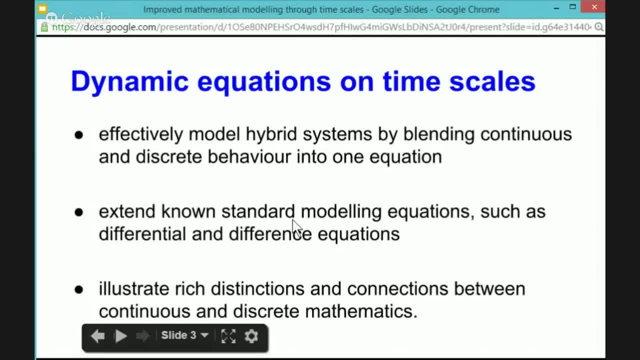 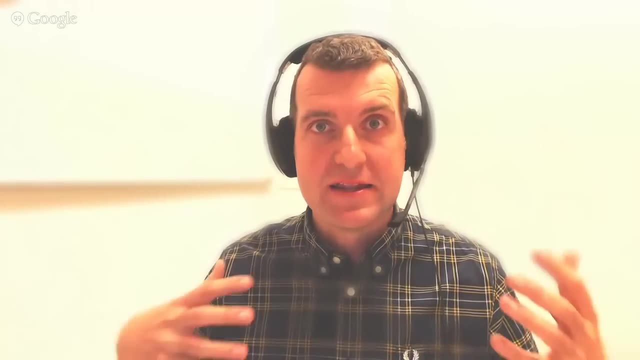 Now, these dynamic equations on timescales also extend the very well-known standard modeling equations, such as differential equations for the continuous problems and difference equations for the discrete problems. So these dynamic equations on timescales, they are more general than these differential equations and difference equations.